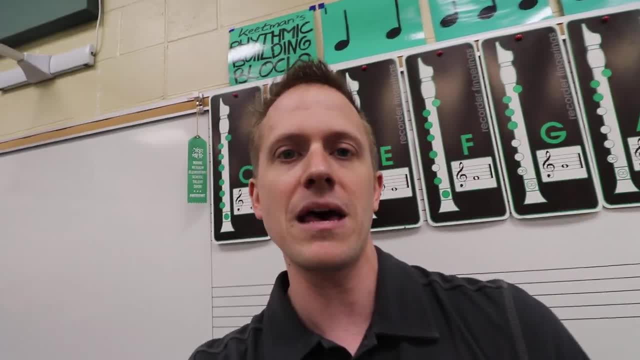 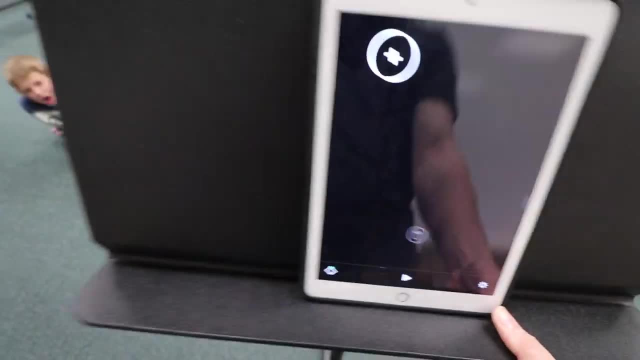 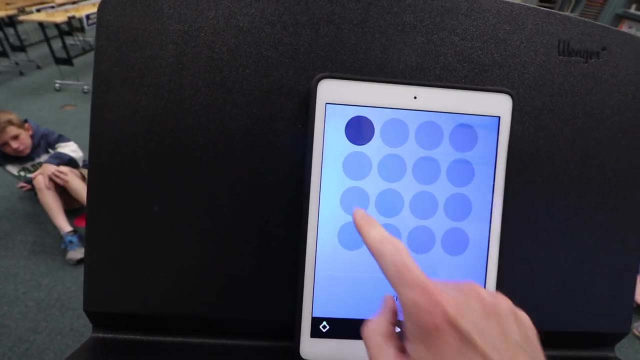 And what I'd like to do is give you a little bit of an idea of how this works and then show you how it can work with my students. So here's the app right here, and all I have to do is push this button to get a kick drum sound, And so I'm going to push some of these circles and push play. 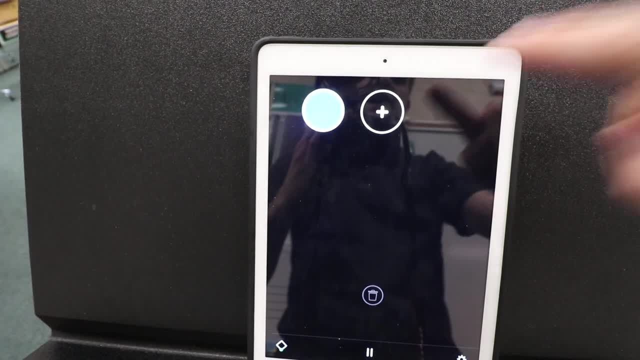 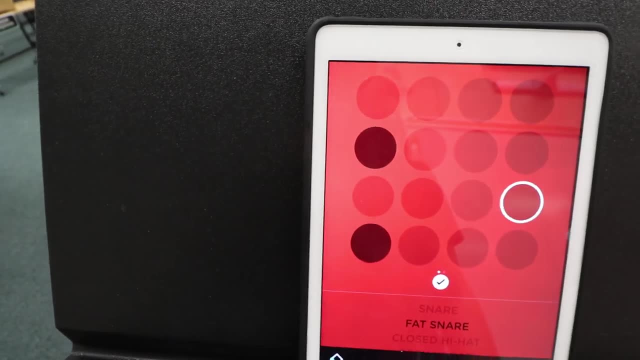 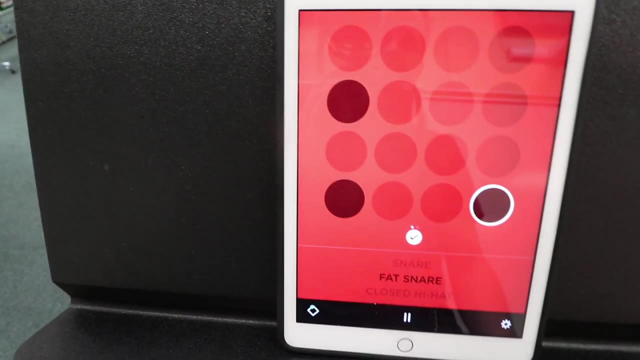 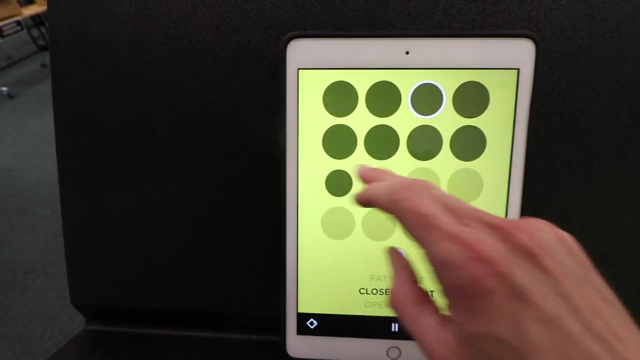 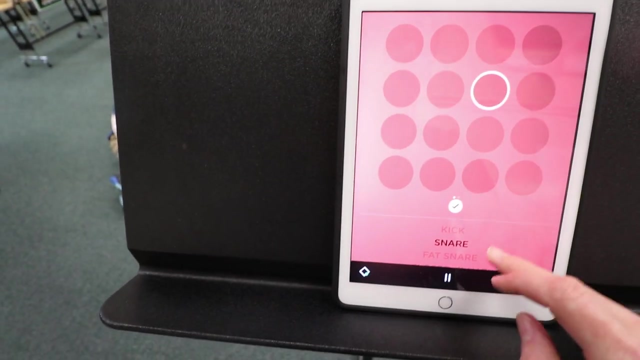 So that sounds pretty cool. And now let's do this. Let's add a snare drum. There we go. That's pretty cool, just like that. I like that. Let's add a hi-hat- There we go. Maybe we'll add an open hi-hat. 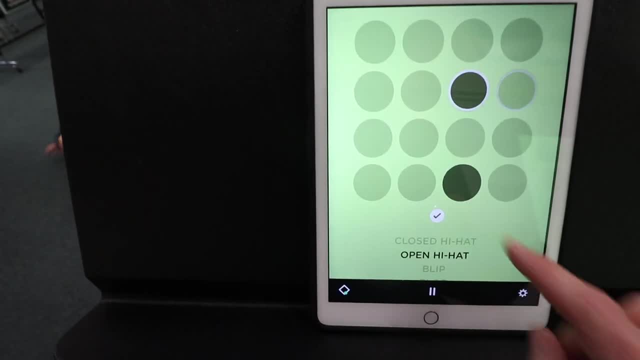 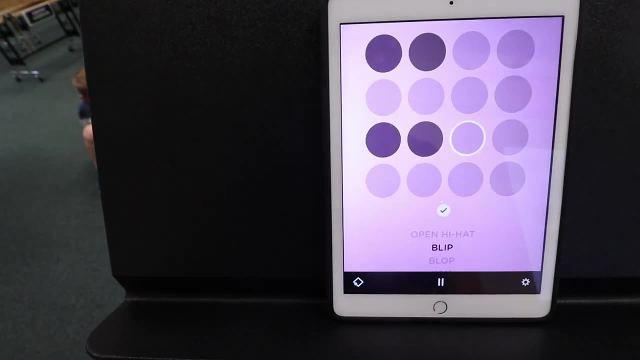 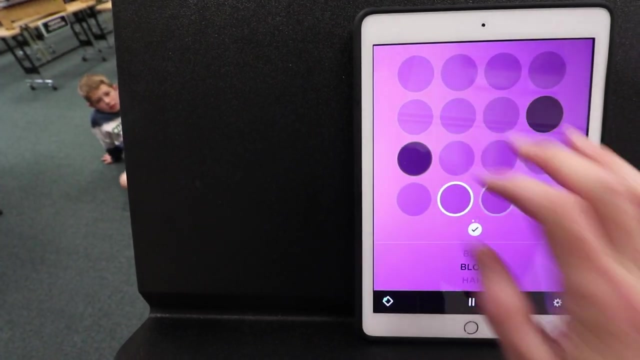 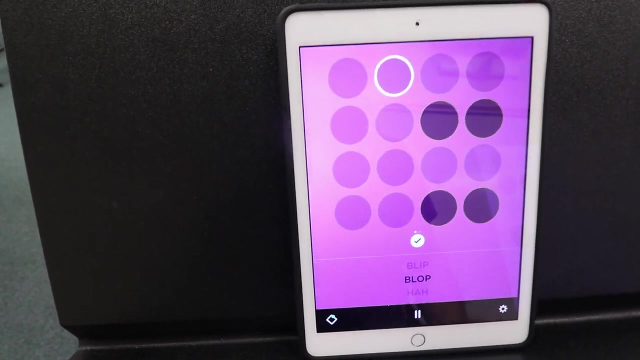 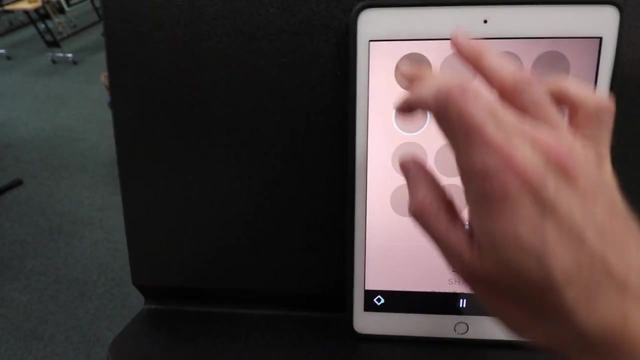 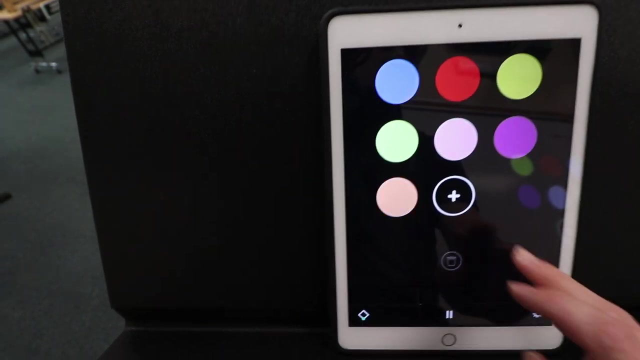 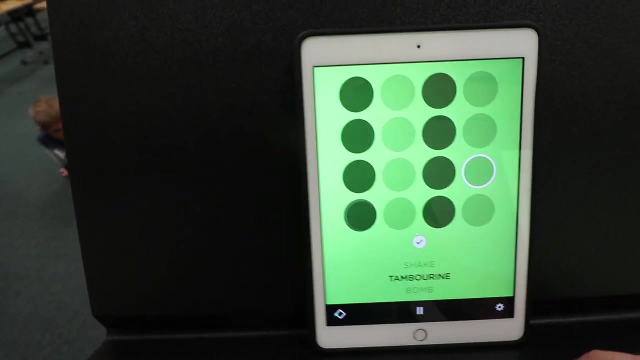 Yeah, that's cool. Yeah, that's cool. Maybe we'll add some blips. We'll add some blops. Yeah, that's cool. Uh, let's some snaps. yeah, just like that. okay, I'll add a tambourine sound. it's pretty cool. 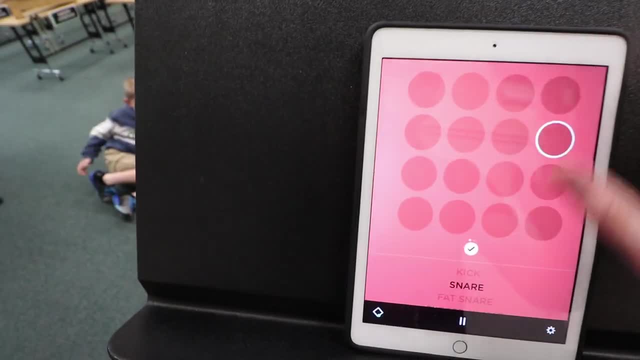 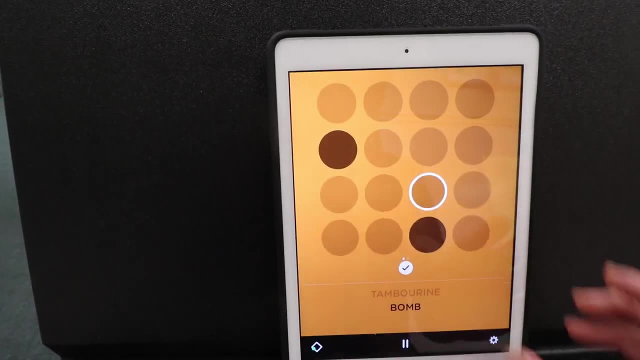 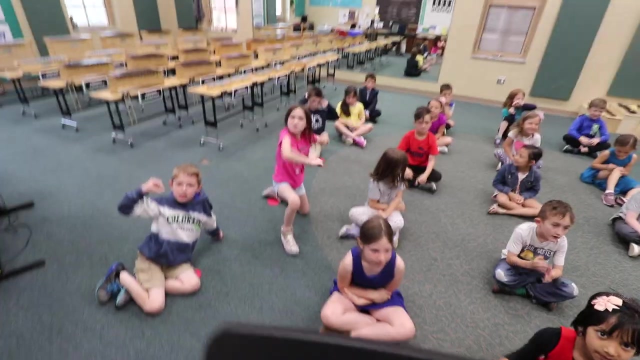 beat now this one. this one's neat. the kids always like this one. it's a bomb sound. all right now, students, are you guys ready to help me? here's what we're gonna do: everybody's gonna get 10 seconds to make a change. 10 seconds, you. 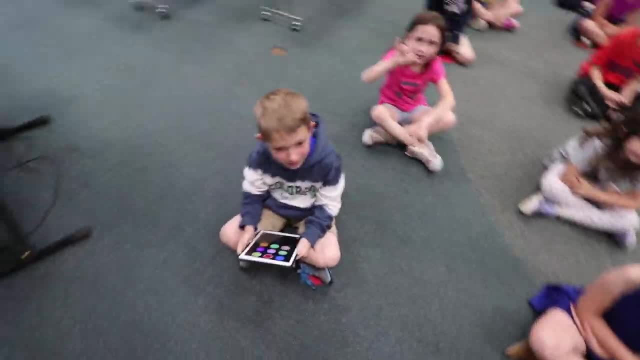 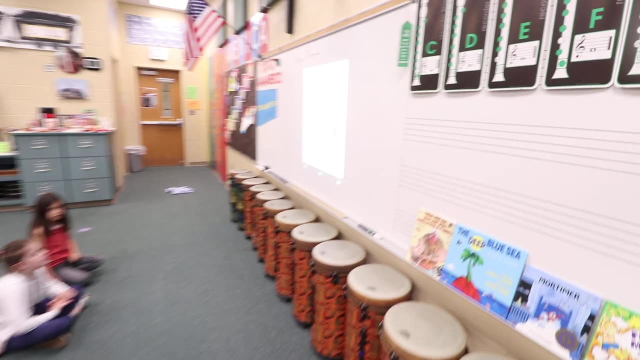 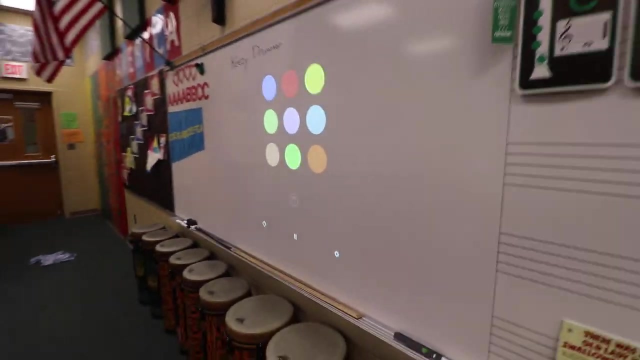 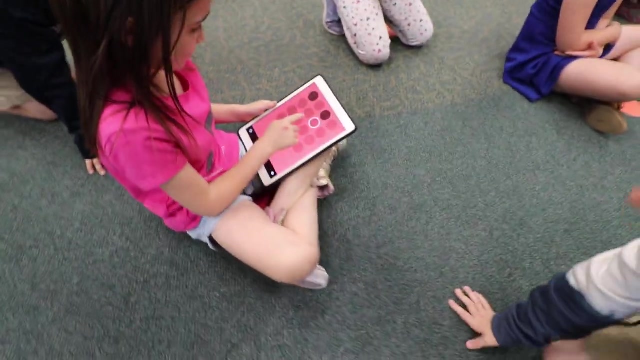 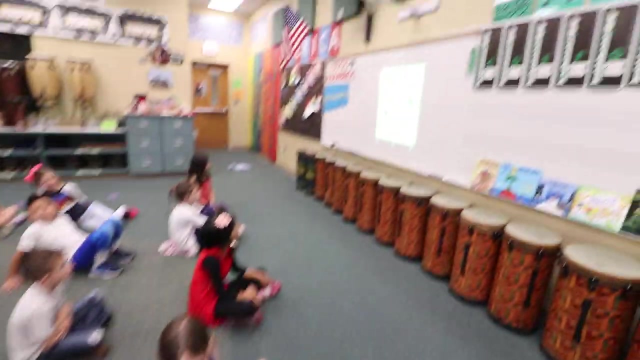 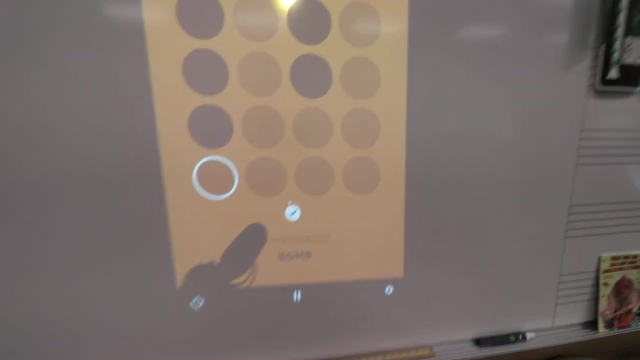 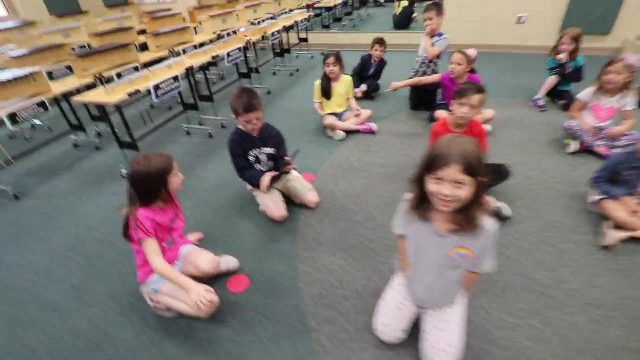 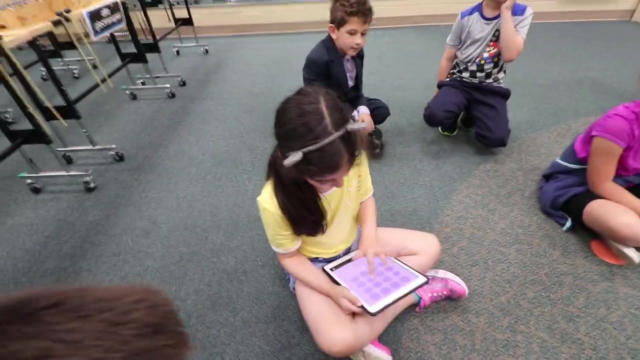 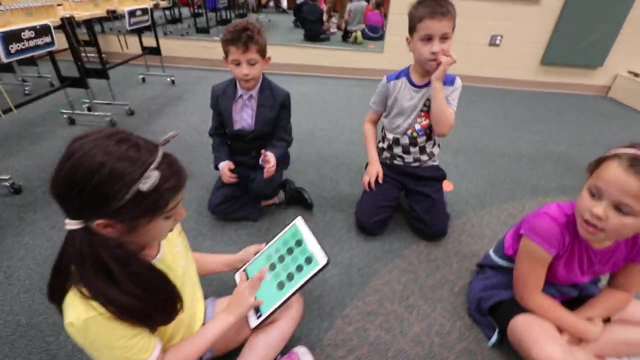 pick your color, make a change and then press the checkmark. go and ten, nine, eight, seven, six, six, five, four, three, two. good, all right, let's pass it on one and go next person. all right, next person, here we go and ten, nine, eight, seven, six, five, four, three, two. one and good, get that checkmark. 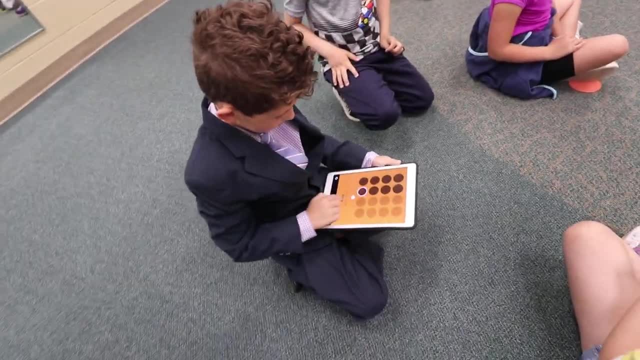 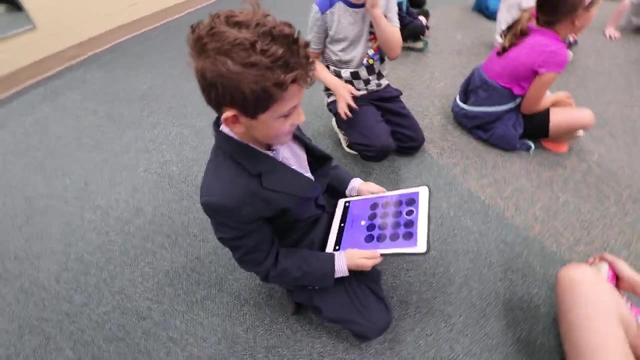 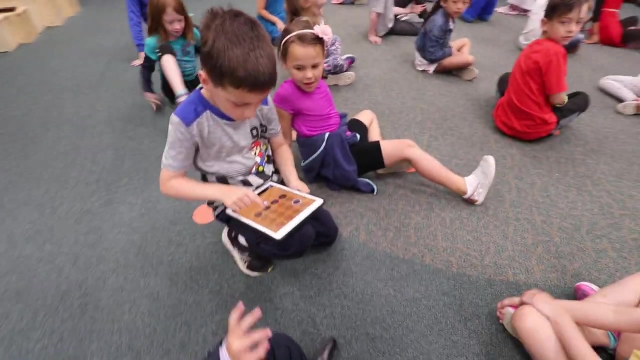 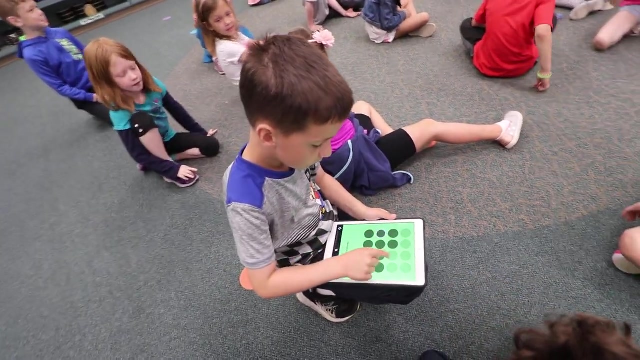 now. we've already got a lot of bomb sound, so maybe do a different one. good, ten, nine, eight, seven, six, five, four, three, two and hit that checkmark. next person. we've already got a lot of those sounds, so let's do something different. there you go, two and one, hit that checkmark. 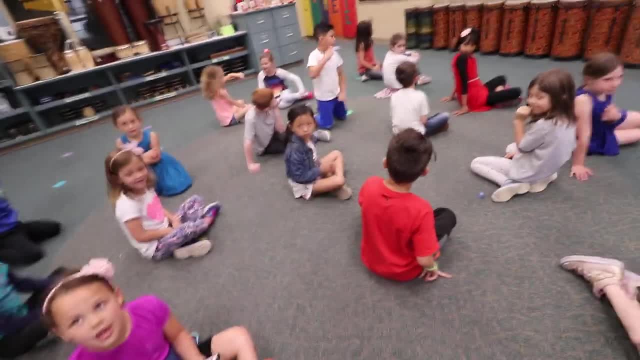 no, no, that's a bad sound. all right, ten, nine, eight, seven, six, five, four, three, two, one and hit that checkmark: 10, 9, 8, 7, 6, 5, 4, 3, 2 1. 10, 9, 8, 7, 6, 5, 4, 3, 2, 1. 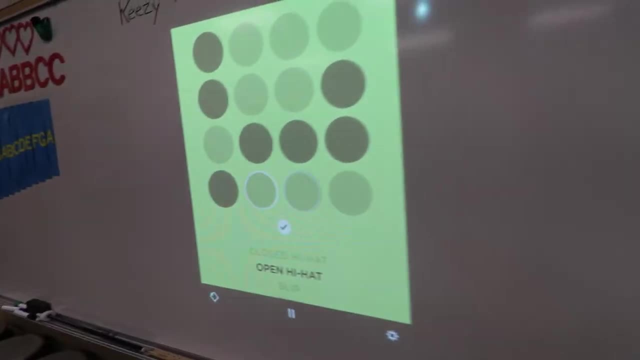 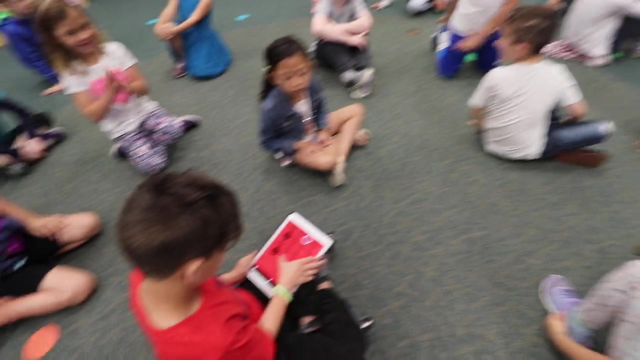 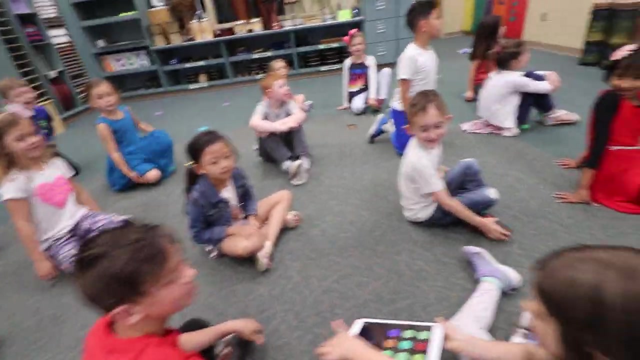 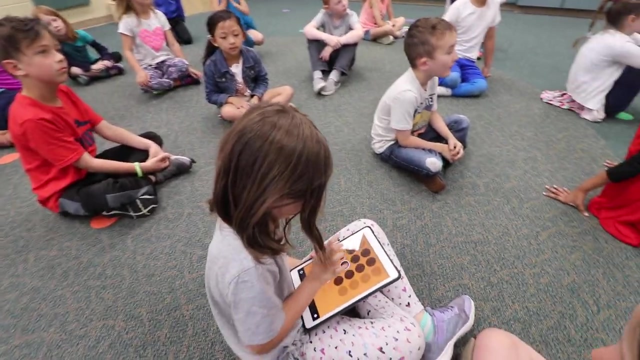 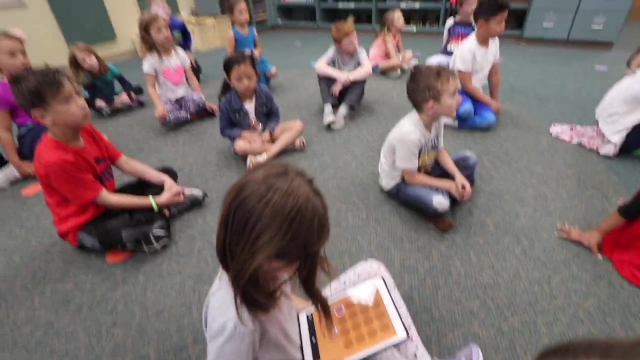 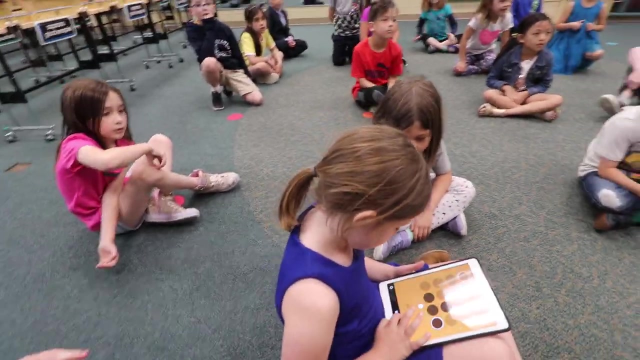 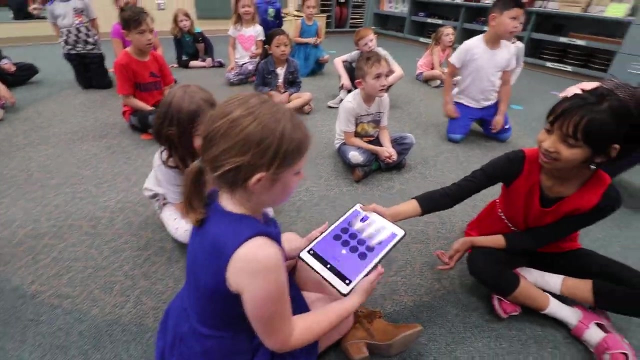 all right, good job, guys, and hit that checkmark. okay, now let's start away from those sounds. so start hitting some of those circles. yeah, good, let's see how it sounds when you take away. good, three, two, one and stop hit that check mark. and three, two, one and check mark. good job, all right, let's take away some of the circles. 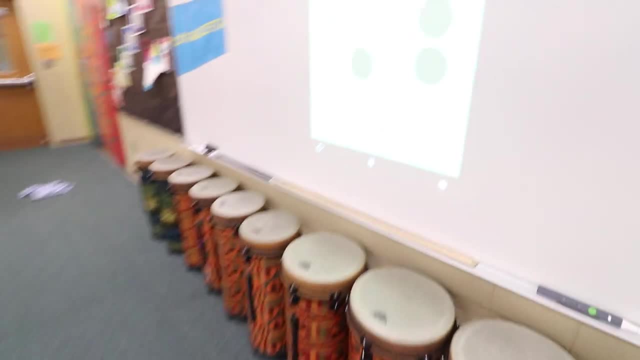 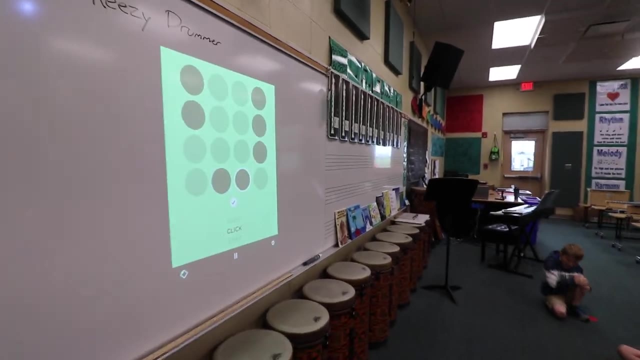 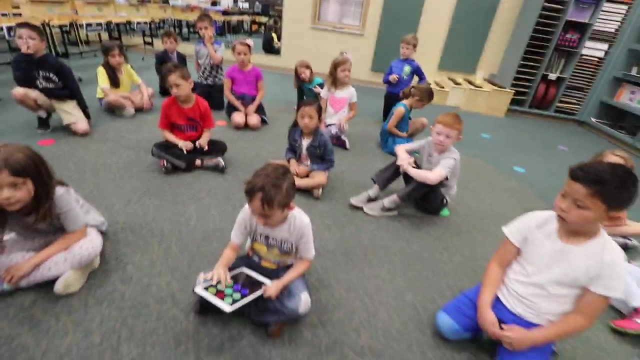 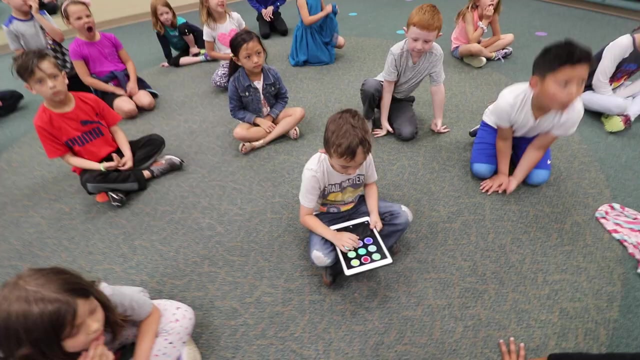 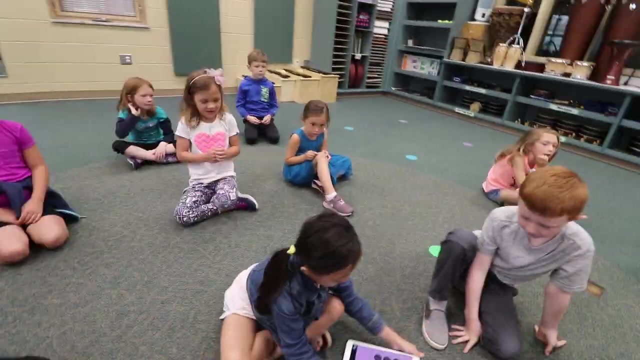 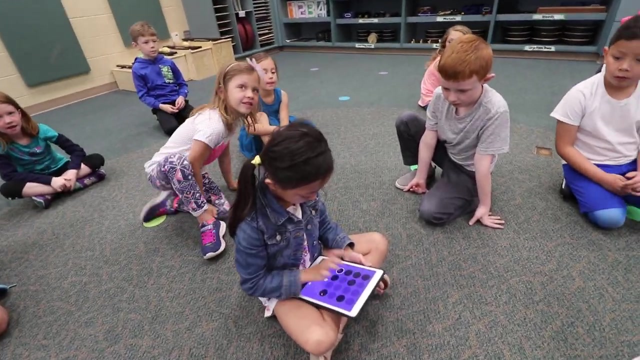 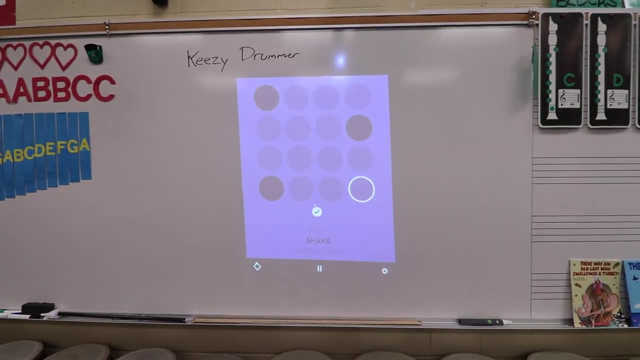 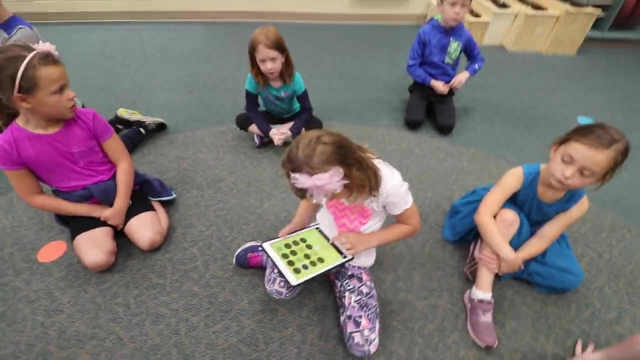 let's hear how it sounds. and three, two, one, good, pass it right back here. there we go. oh, listen to how that changes the music. yeah, great. three, two, one and stop. good to back, excellent, good. so now we're getting rid of some of our sounds and our beat is changing a little bit. 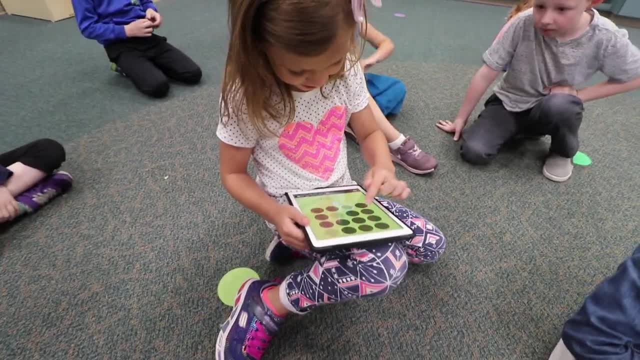 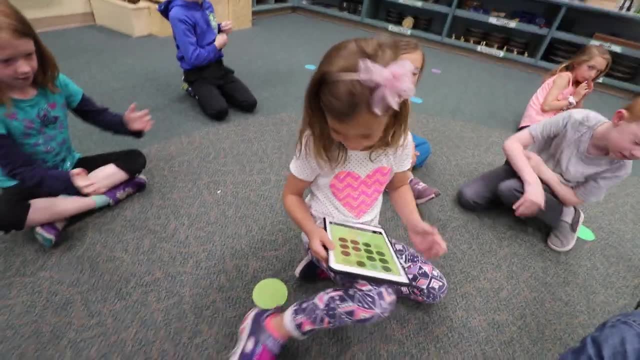 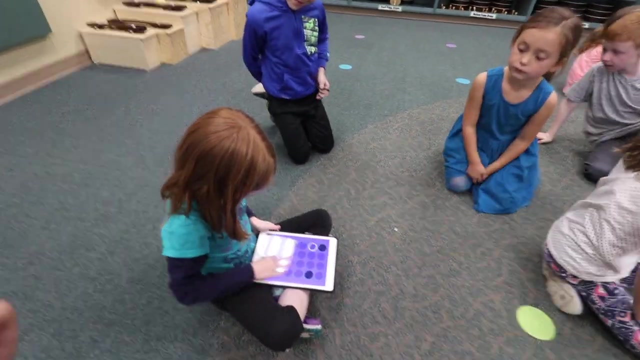 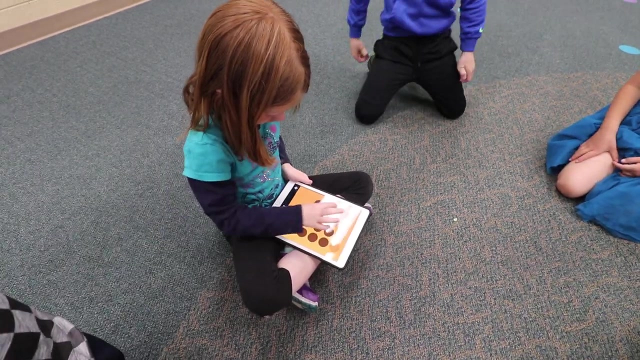 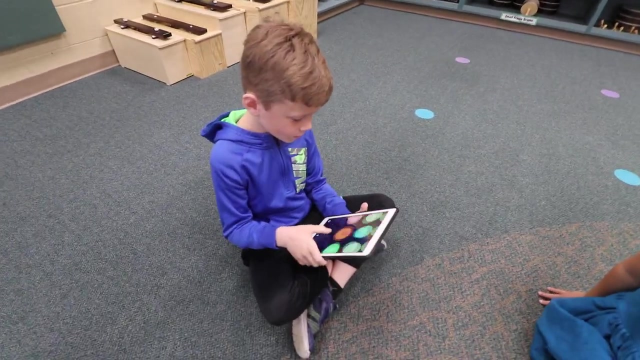 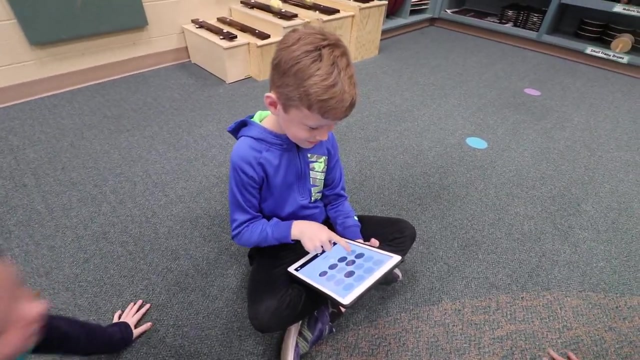 cool. oh, i like that, don't you guys like that? three, two, one and pass, nice job. hit that check mark. yep, good, now you can pick any color. and three, two, one and stop. okay, hit that check mark, let's see what we're doing. and five, four, three, two, one, nice job. 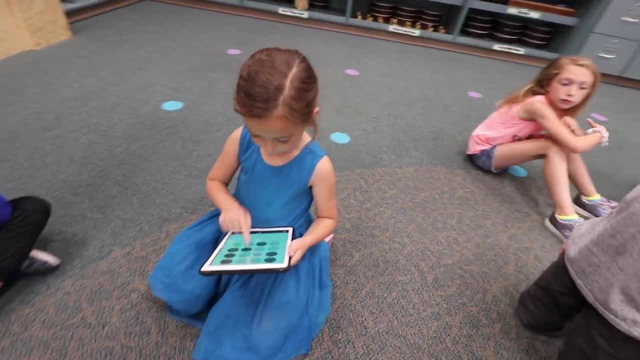 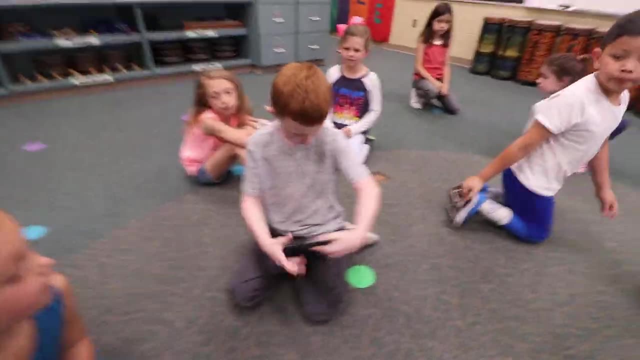 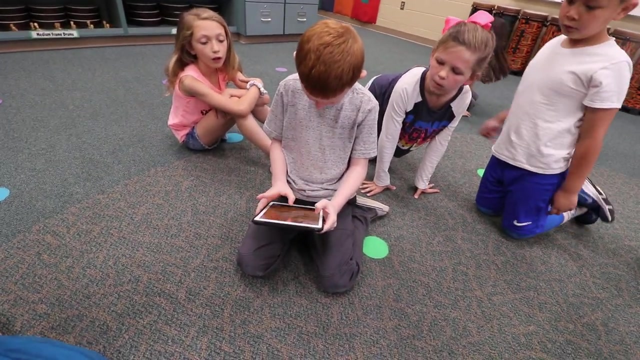 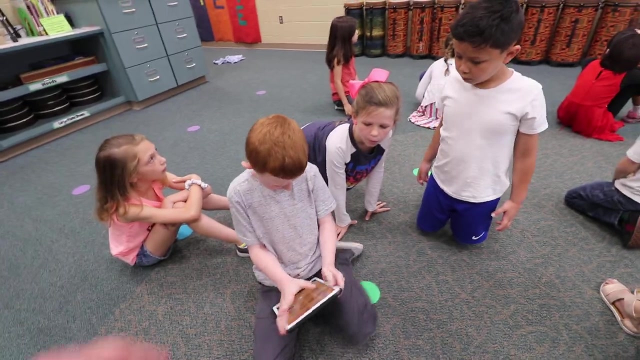 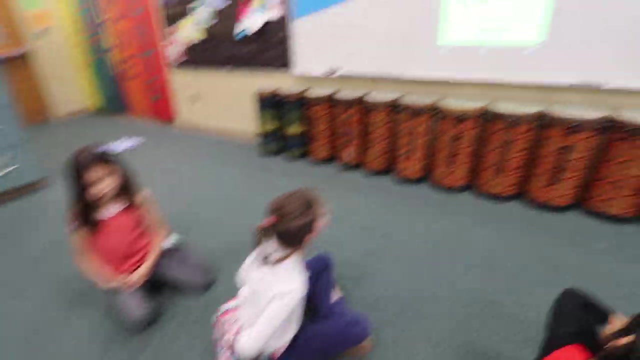 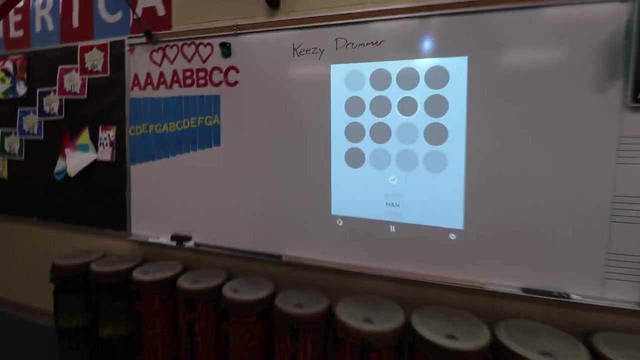 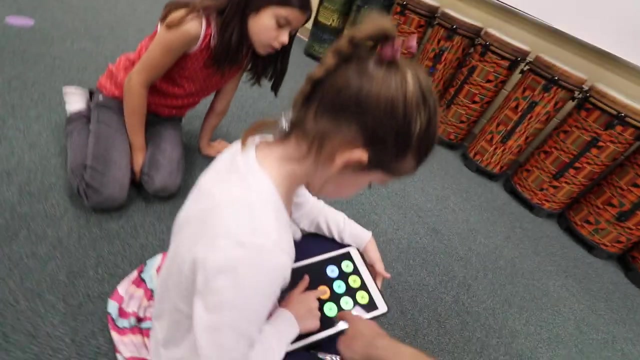 ten, nine, eight, seven, six, five, four, three, two, one and stop. great work. okay, let's try and take out some of those ones on the orange, all right. and ten, nine, eight, seven, six, five, four, three, two, one and stop. 10,, 9,, 8,, 7,, 6,, 5,, 4,, 3,, 2, 1, and stop Good 10,, 9,, 8,, 7,, 6,, 5,, 4,, 3,, 2,. 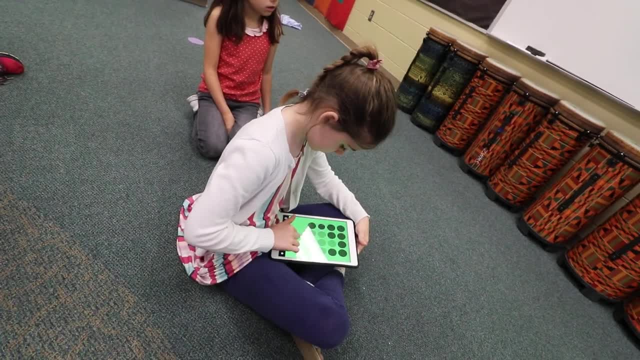 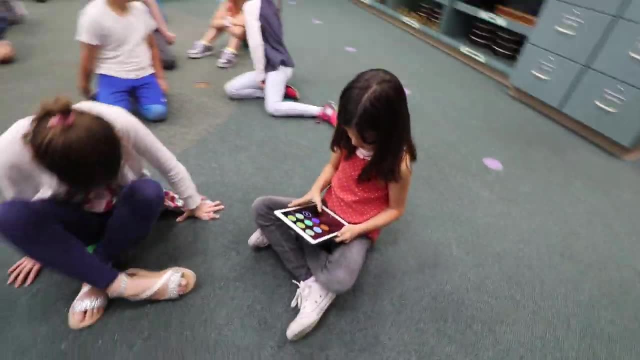 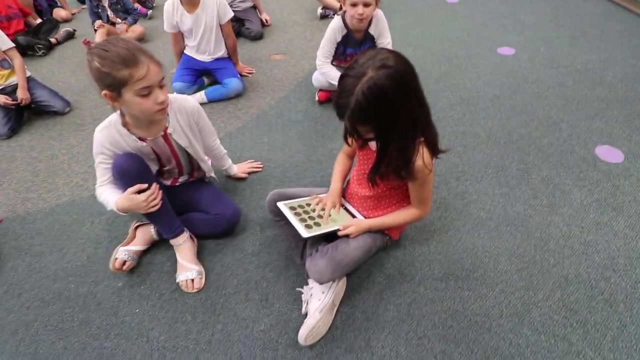 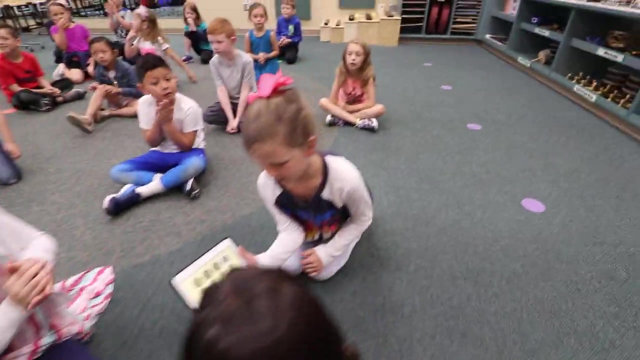 We'll give you a couple more seconds: 5, 4,, 3,, 2,, 1, and stop, Nice, Pass it on 9, 8, 7.. Ooh, that's cool with the clapping sound. I like that. 5, 3,, 2, 1, and 10,, 9,, 8,, 7,.